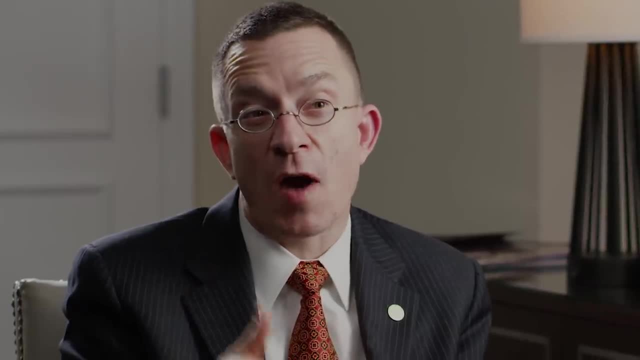 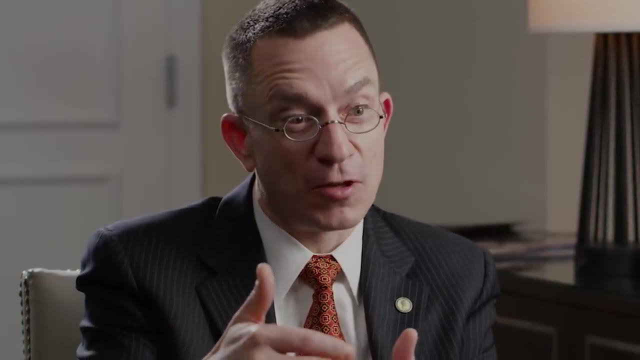 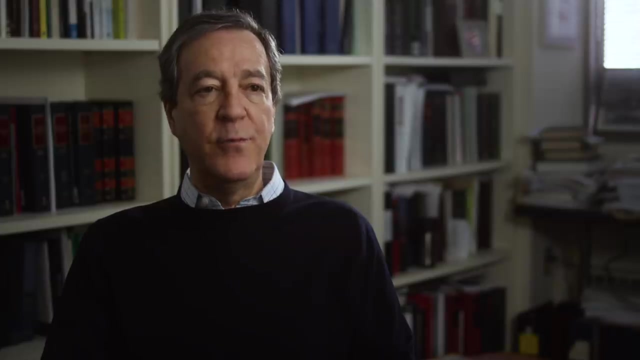 water is. That becomes important because the agencies have to know how far can they regulate. They can regulate no farther than under the Clean Water Act, than in regulating discharges into navigable water. The term navigable waters originated in an entirely different context in terms of defining. 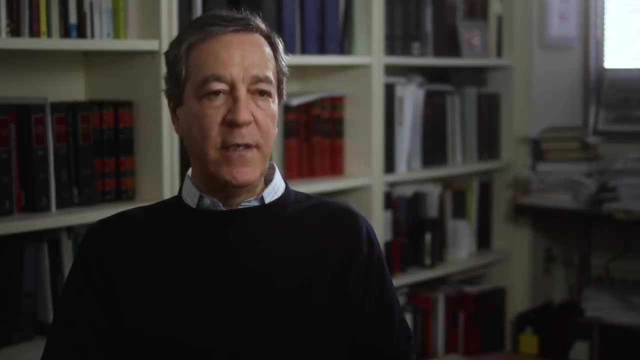 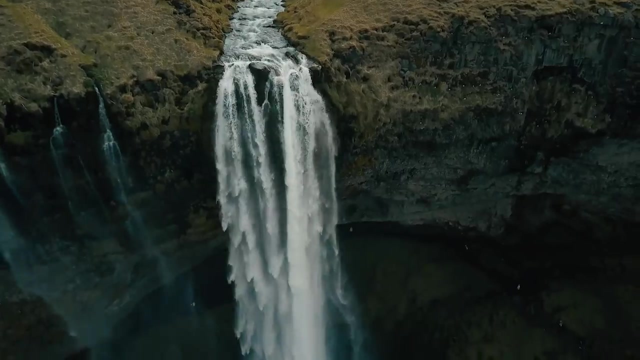 the scope of the federal government's constitutional authority to regulate certain activities that relate to water. The idea there was, in part, to make sure that rivers, lakes and streams remained navigable so that river traffic could proceed down those waters. There is a stark difference between what some people consider to be navigable waters and what the 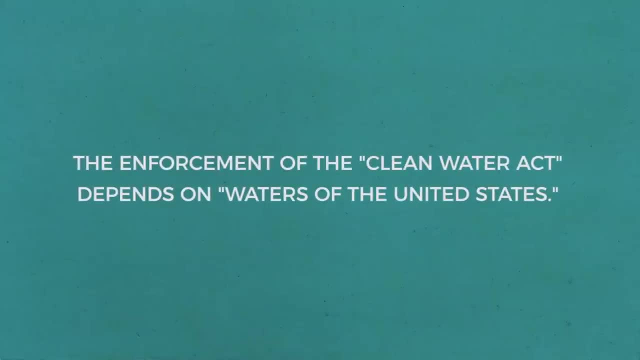 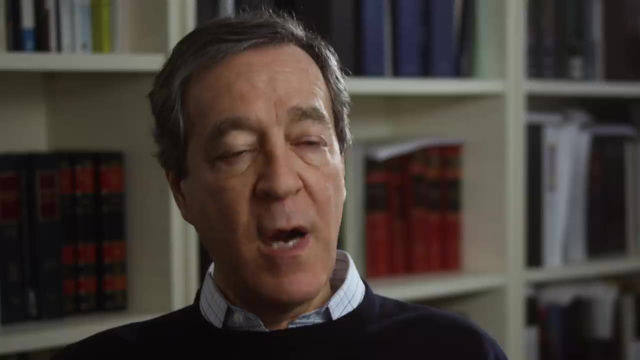 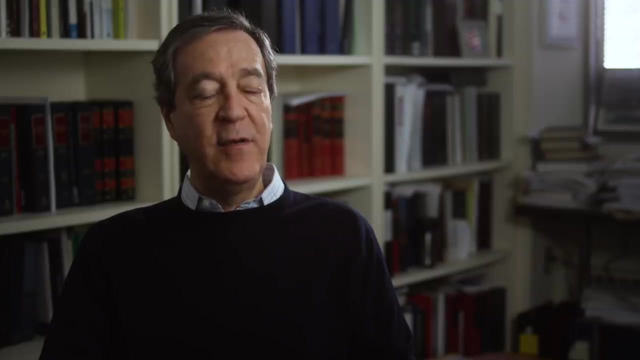 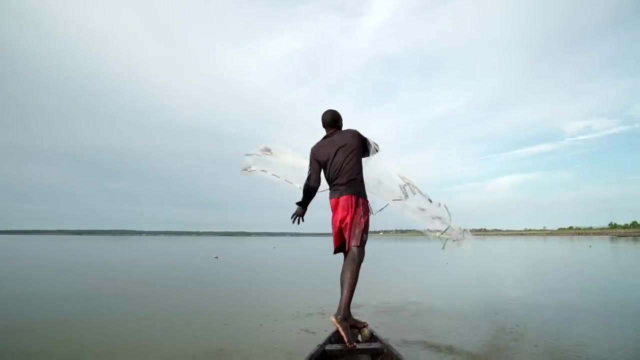 statute is designed to cover. The operative term really is waters of the United States, not navigable waters. Congress was trying to ensure that a broad range of waters and wetlands were protected, Basically, anything that could affect the environment, That could affect the integrity of the hydrological cycle And the reason we want to protect. 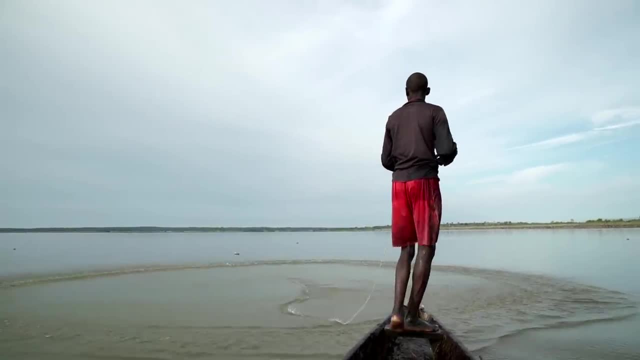 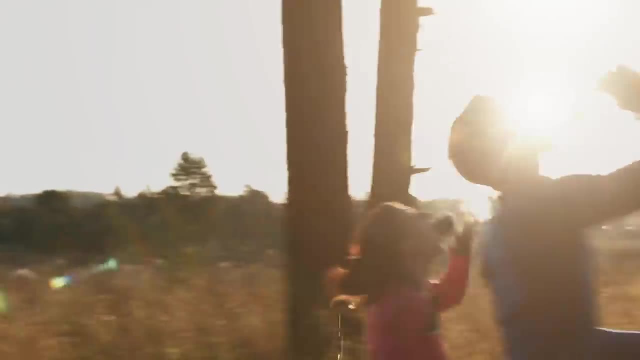 the chemical, physical and biological integrity of waters in the United States is number one. people may drink that water. We don't want people drinking polluted water. that creates hazards to their health. Even if they're not drinking the water, they may expose themselves. 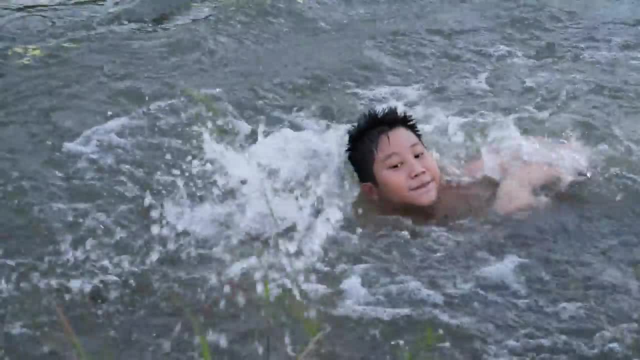 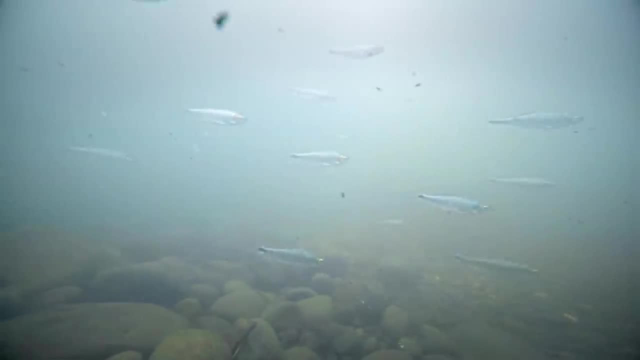 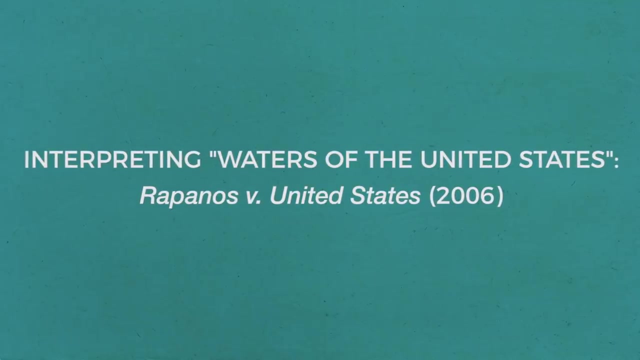 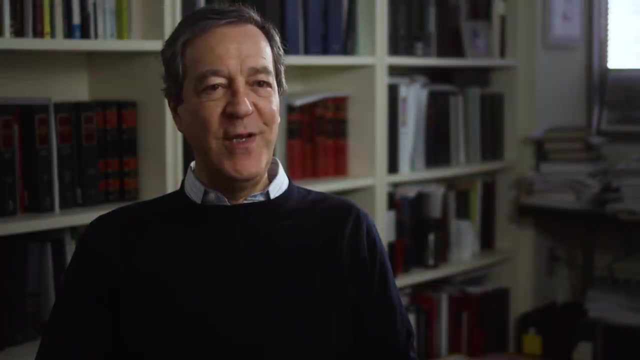 or encounter the waters for recreational purposes. And again, if the water is polluted, that exposure creates a public health risk. Finally, even if people are not directly using the water, the water is often integral to the integrity of some ecosystem. There was no precedent for what waters of the United States means, given that it was. a newly created term in 1972.. And so EPA and the Court of Engineers had to figure out what Congress meant by waters of the United States. They issued regulations in the 1980s which have been amended several times since then, And so we have the Raponos case in the mid-2000s, in which the US Supreme Court, through a 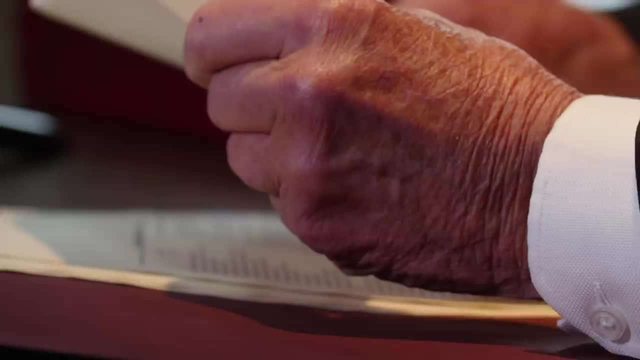 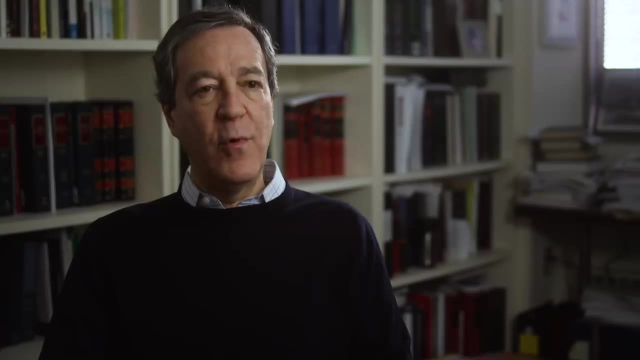 variety of plurality opinions tried to determine whether or not the EPA's then definition of navigable waters was satisfactory. Kennedy's opinion said that a body of water qualifies as a water of the United States if there is a significant nexus between a body of water and a body of water of the United. 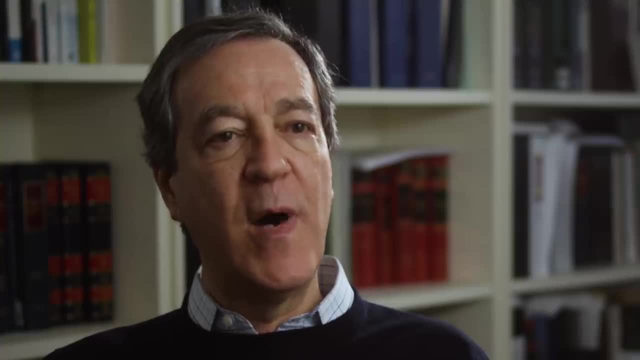 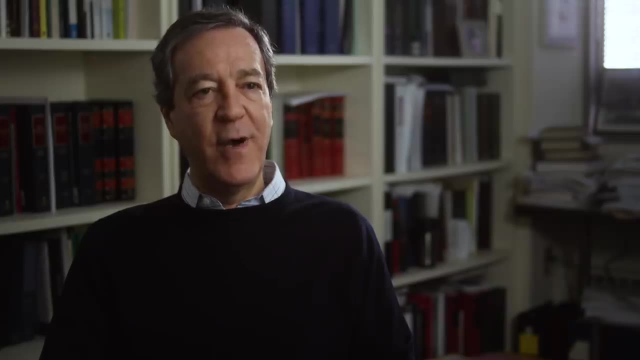 States A body of water or a wetland and a traditionally navigable body of water like a lake or a stream or a river. The significant nexus test is designed to identify those bodies of water or wetlands which are not, per se, covered by the rule whose pollution will or might adversely affect. 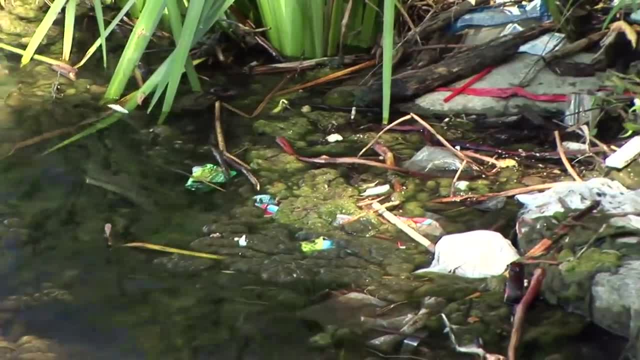 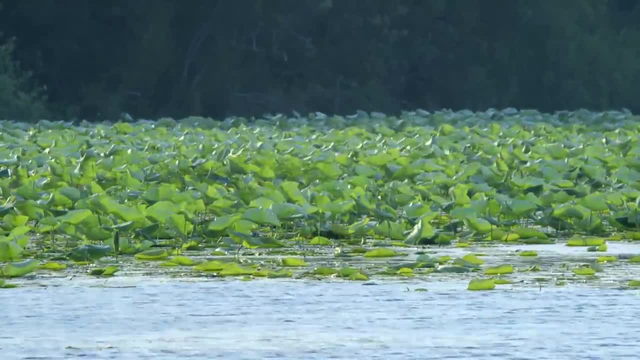 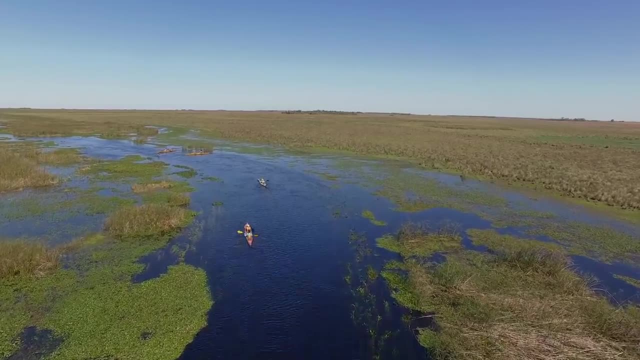 the chemical, physical or biological integrity of a water of the United States That might be a wetland, for example, That is not directly adjacent to a river, a lake or a stream, but that has some impact on the quality of the water in those bodies of water or wetlands. 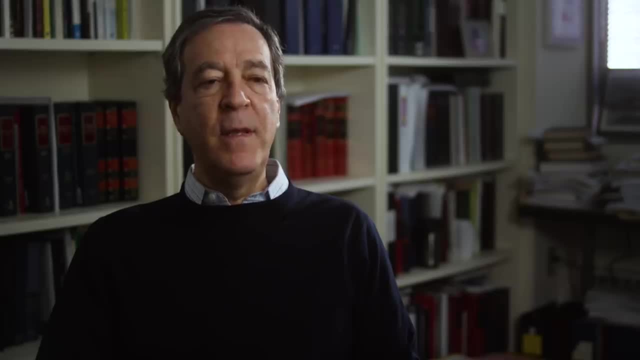 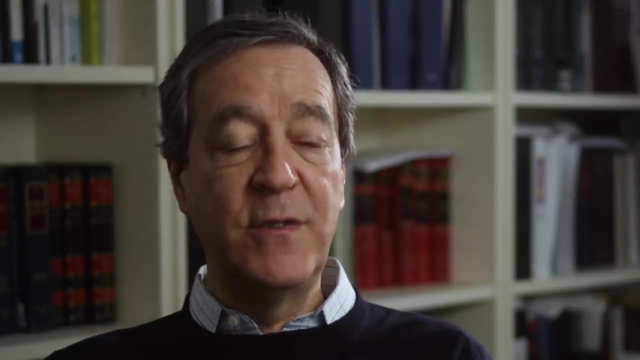 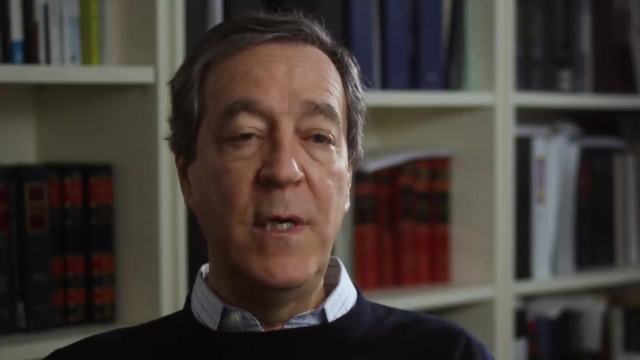 Chief Justice Roberts, in a separate opinion, urged EPA and the court to amend their regulations defining water of the United States, because the definition was unclear and created uncertainty for everybody: For the agencies, For regulated parties, For those who benefit from regulation, For those who don't. 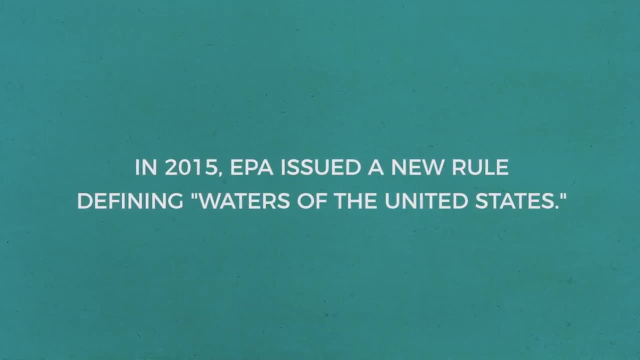 For those who are afraid to be part of regulation, For those who are afraid to be part of regulation, For those who are afraid of regulation, For those who are afraid of regulation, For those who are afraid of regulation And those who are afraid of regulation. That broad ruling of course raised a lot of controversy. In order to get a permit to discharge into the water of the United States, it can sometimes take two. I think the average is something like $250.. like 270 days from the application period to afterwards. 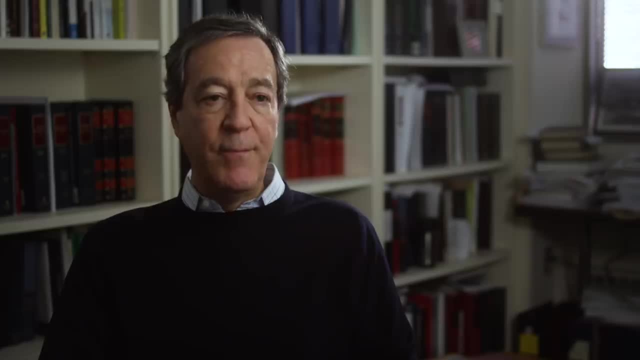 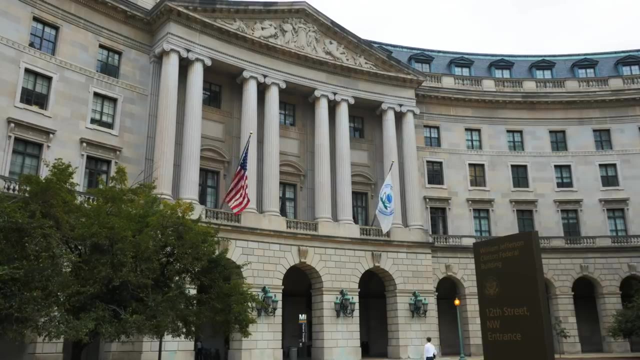 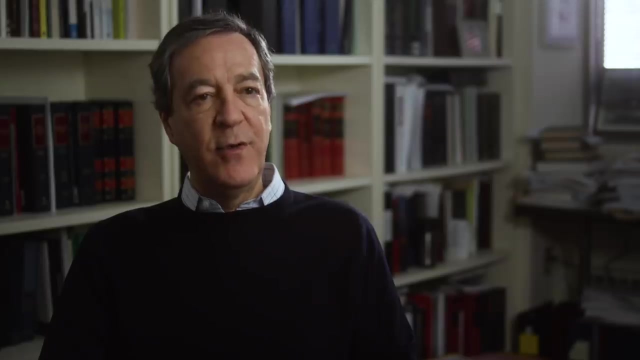 With the dredge and fill permit program where you have a private property owner who wants to develop or build on the land. the land contains some wetlands and the agencies say, well, you can't fill these wetlands as a first step toward developing the lands, unless you 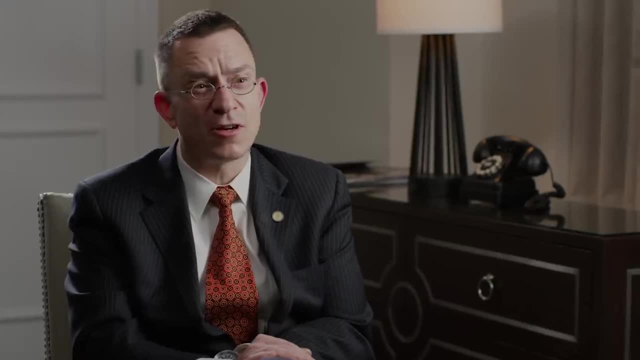 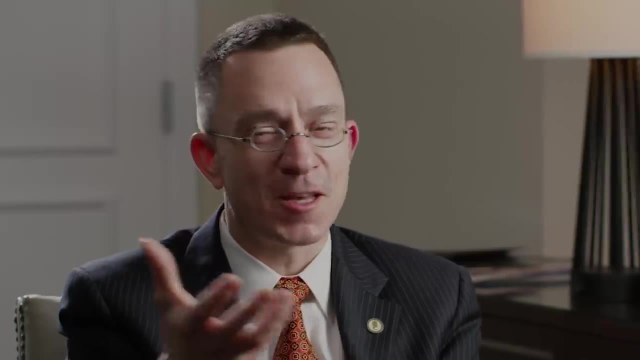 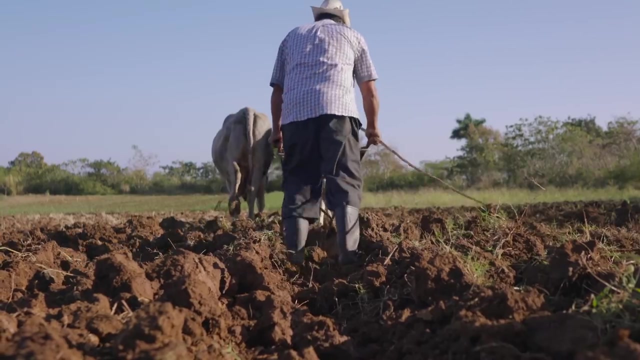 first get a permit from the Corps of Engineers. It's a substantial cost to individuals, who each are spending hundreds of thousands of dollars. sometimes We're talking about the family-owned farm who happens to have a ditch 100 miles away from a river that is now potentially ensnared in this process. 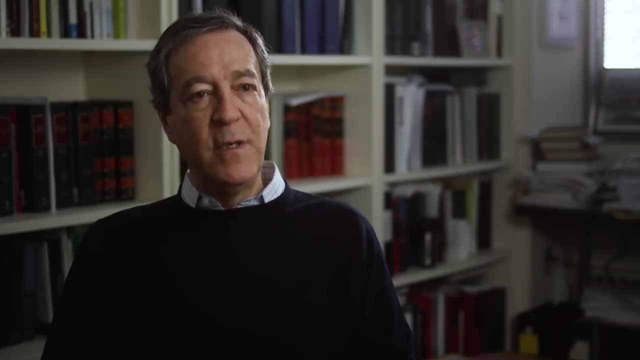 But even if you believe that the regulation did at least something to clarify the scope of the Clean Water Act's coverage, there are those who believe that the regulation is too expansive and that it covers too many waters, waters not intended to be covered by Congress.